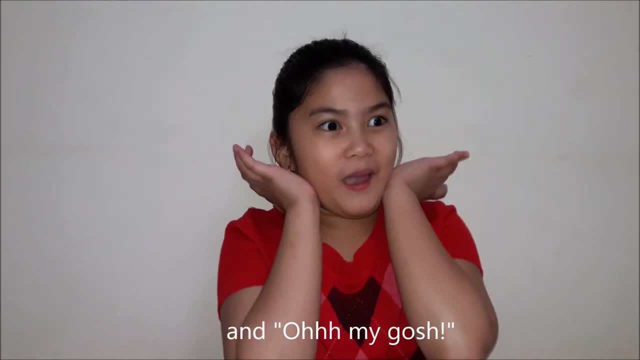 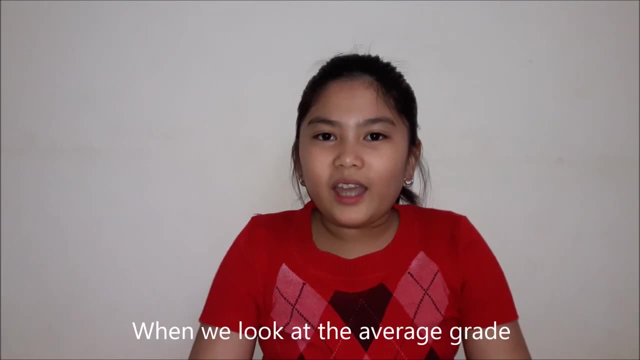 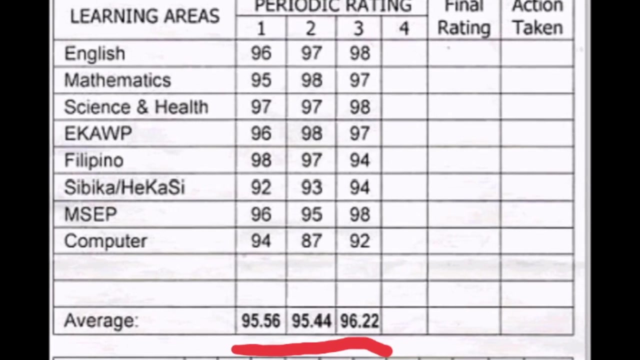 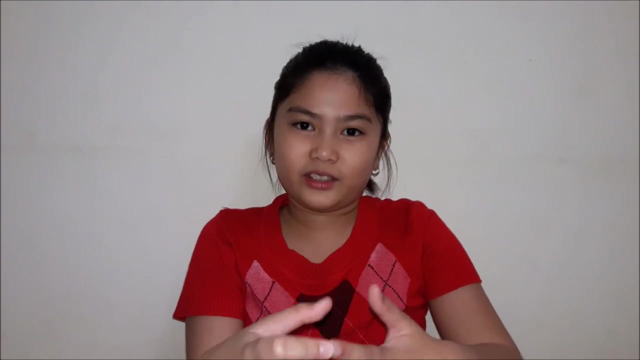 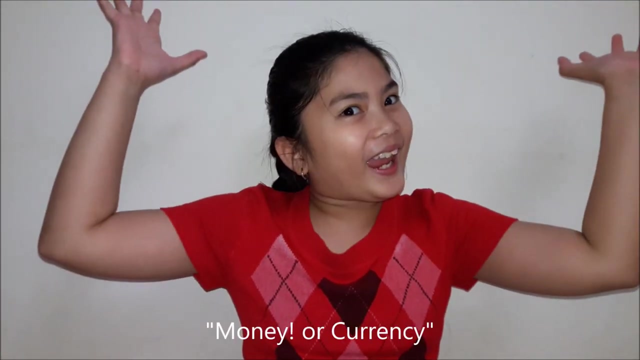 And then when you weigh yourself, and oh my gosh, you weigh 30.50 kilograms. When we look at the average grade on our report cards, we sometimes see decimals. At the gasoline station, the prices are also reflected as decimals. Last but not the least, of course, money or currency. In the Philippines it is called centavos, but in the UAE it is called centavos. 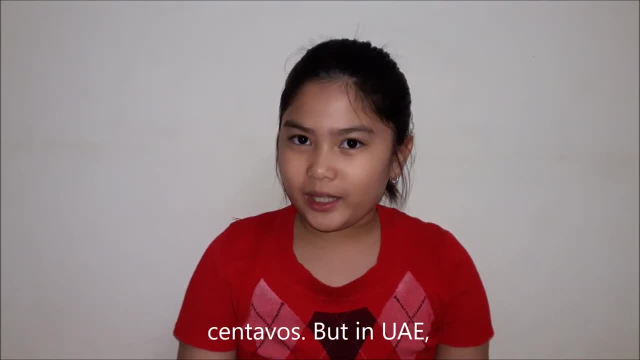 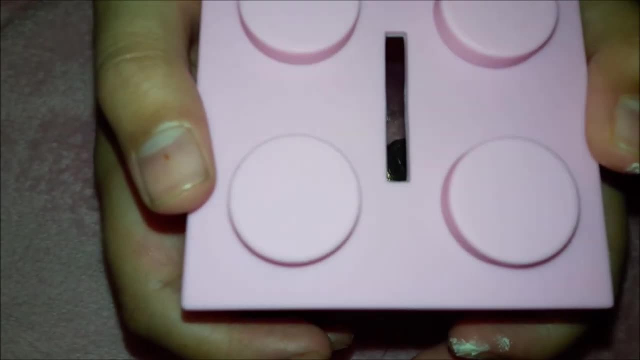 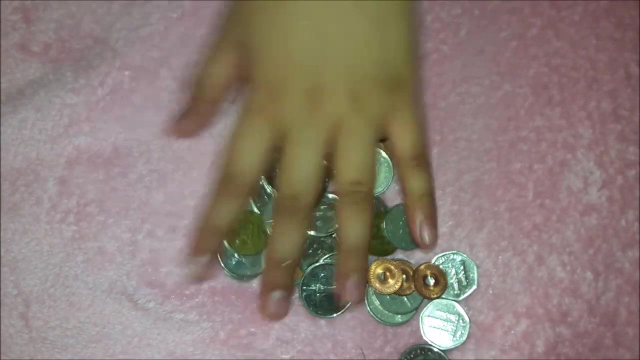 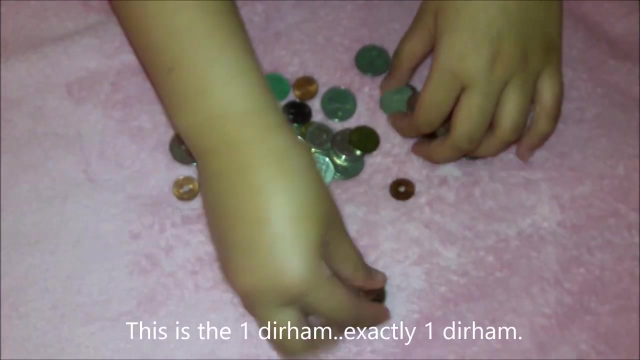 In the Philippines it is called centavos, but in the UAE it is called centavos, It is called bills. Let's open my Lego Bank. Okay, let's sort this out. This is the Wonder Home, Exactly Wonder Home. 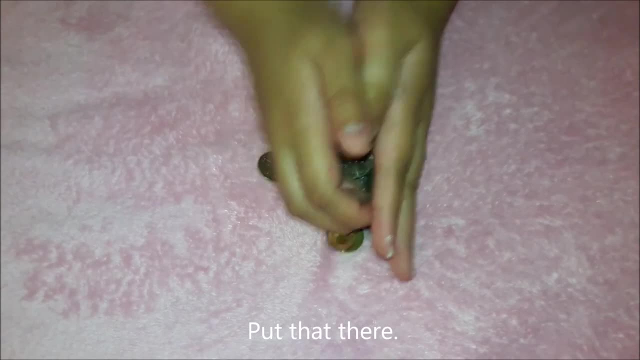 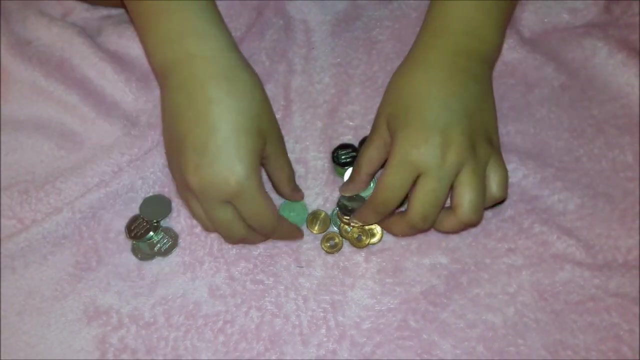 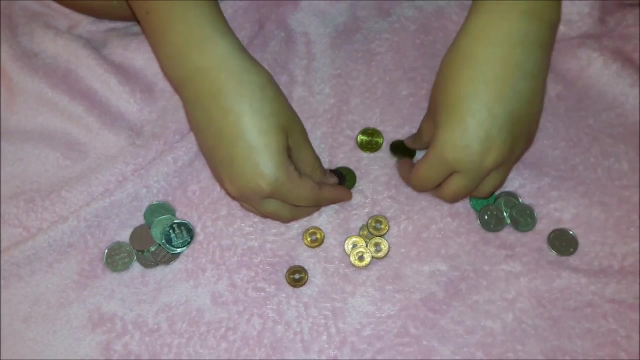 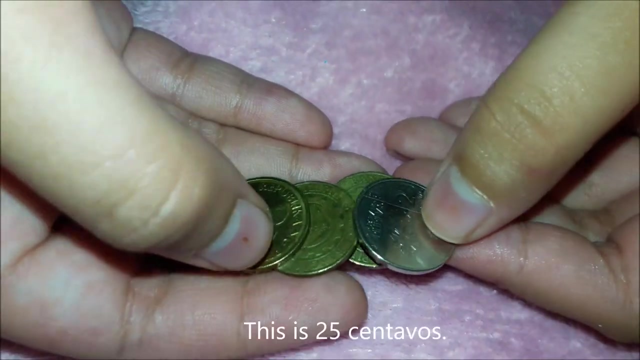 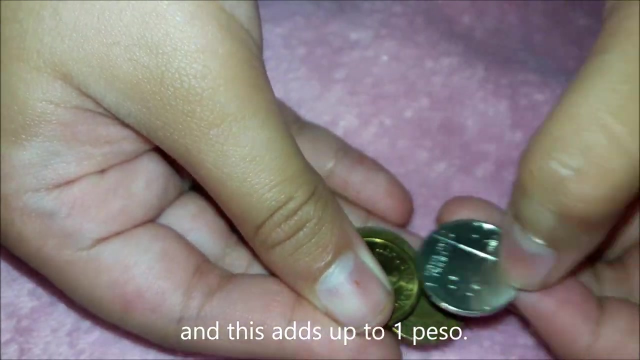 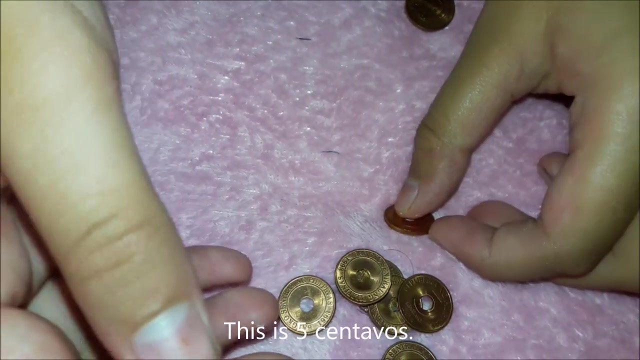 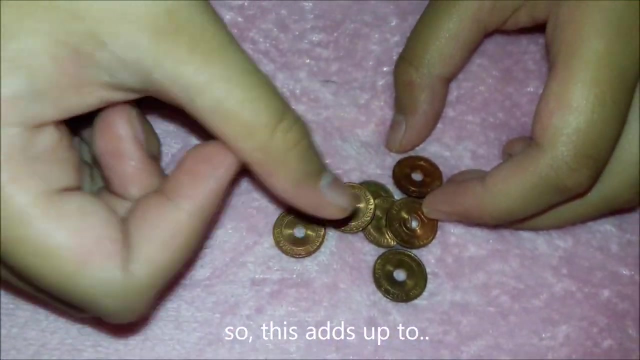 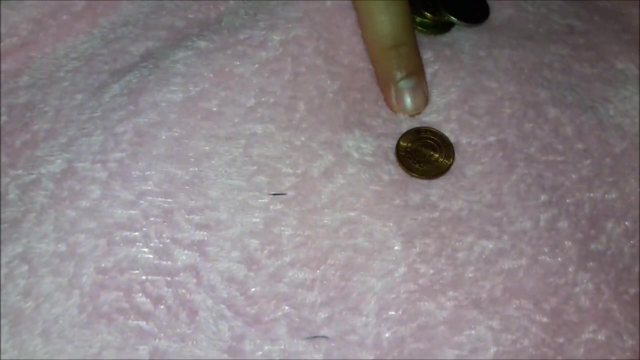 Okay, let's insert this again. This is 25 centavos. This is for 2018.. And this adds up to 1 peso. This is 5 centavos. As you can see, there is a hole, So this adds up to 35 centavos. 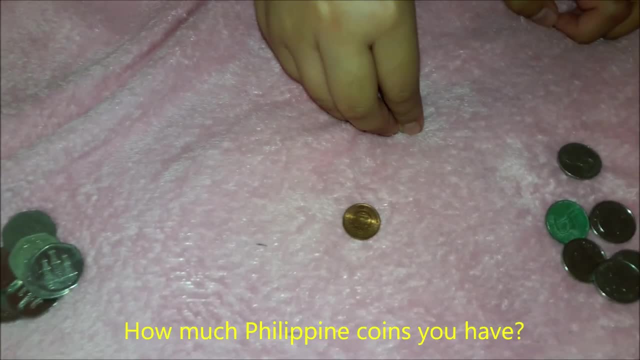 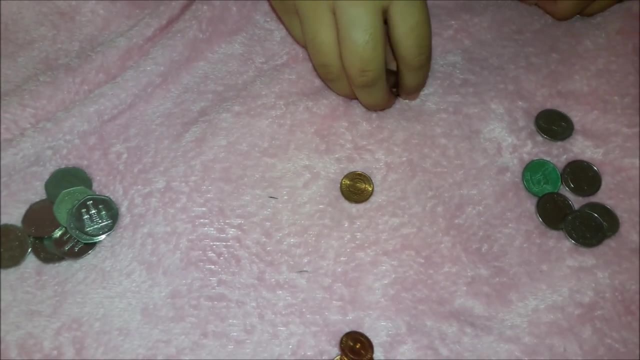 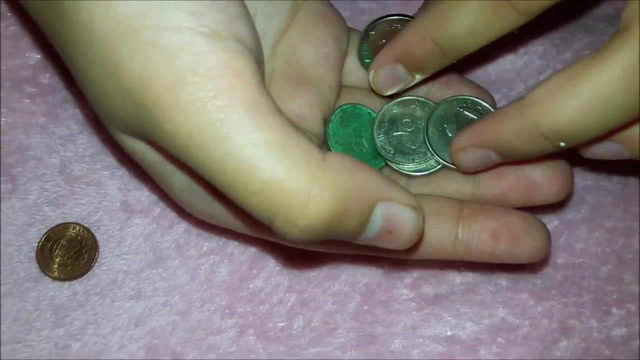 This is 10 centavos. 1.45.. This is 25 phils. This adds up to 1 dirham and 50 phils, And this adds up to 10 centavos. This is 10 centavos. 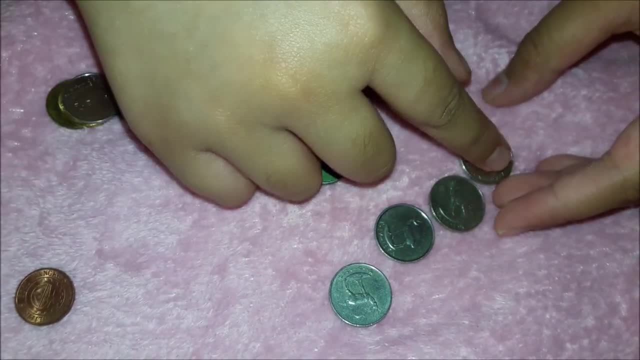 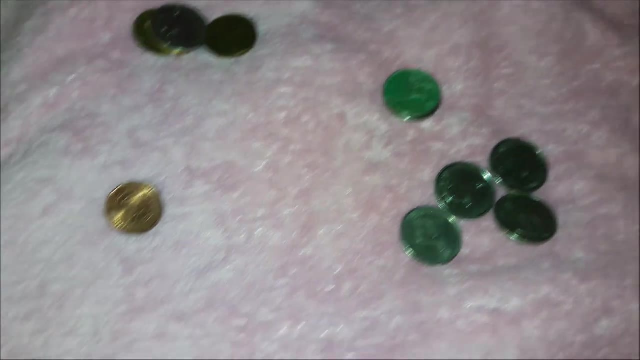 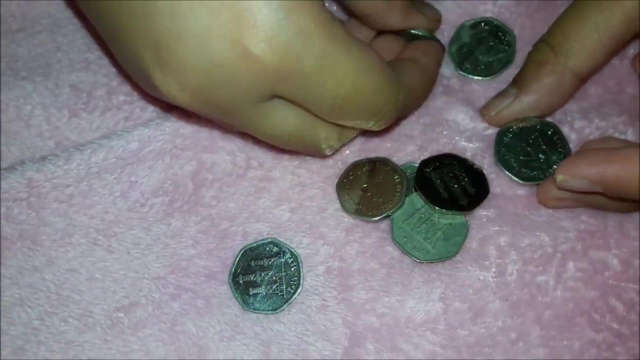 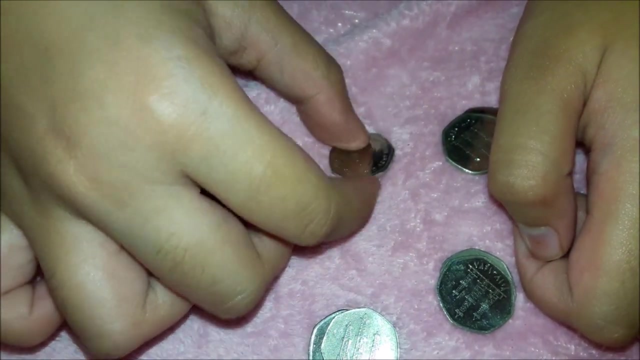 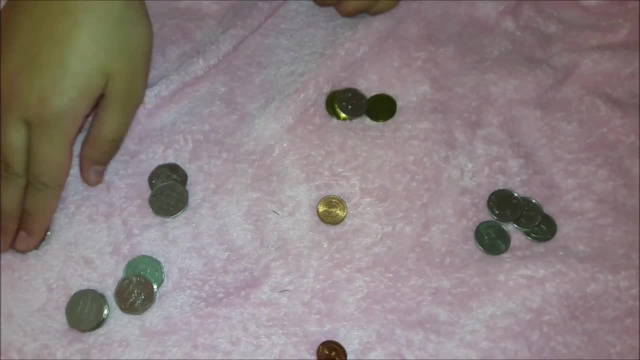 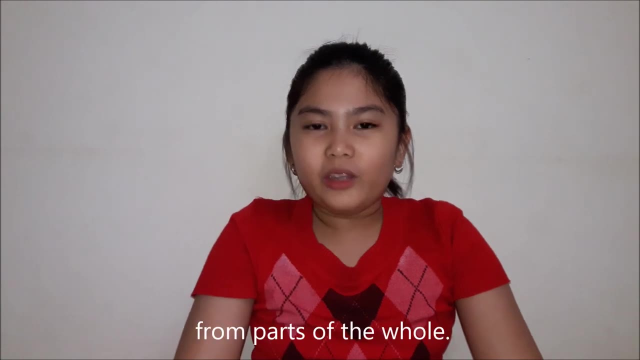 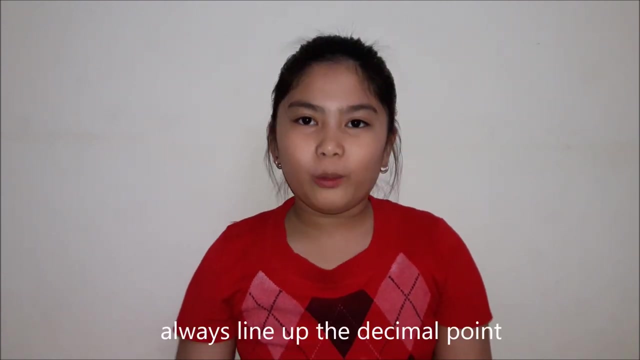 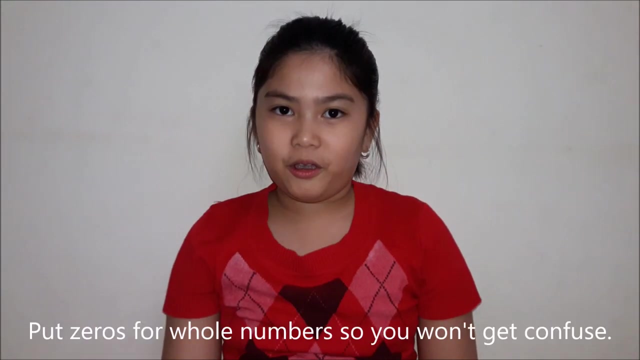 Added up together equals 6 dirhams. The decimal point separates the whole number from parts of the number- the whole. so remember, when adding or subtracting decimals, always line up the decimal point using a column. addition or subtraction, put zeros for whole numbers so you won't get confused, and always remember to put the decimal point in the 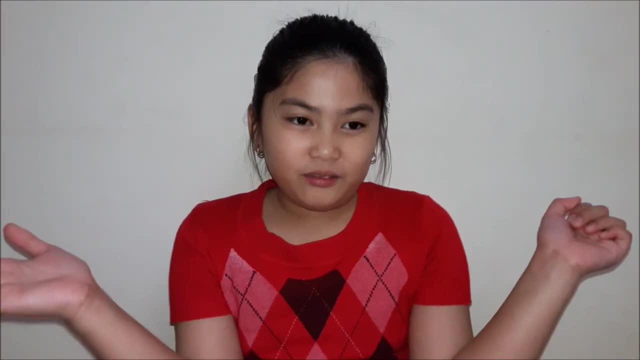 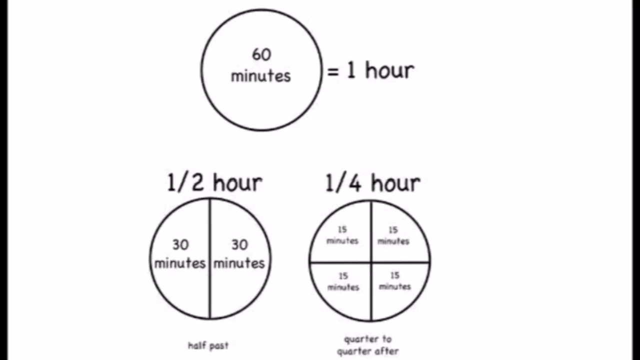 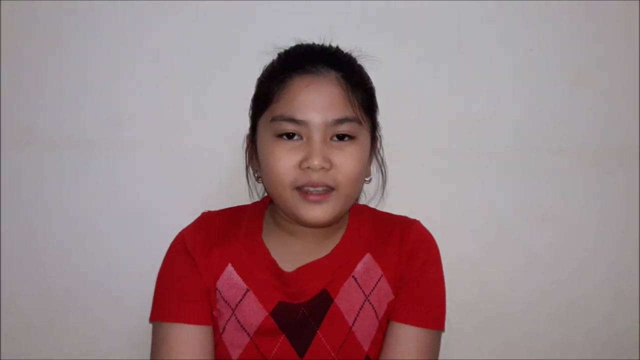 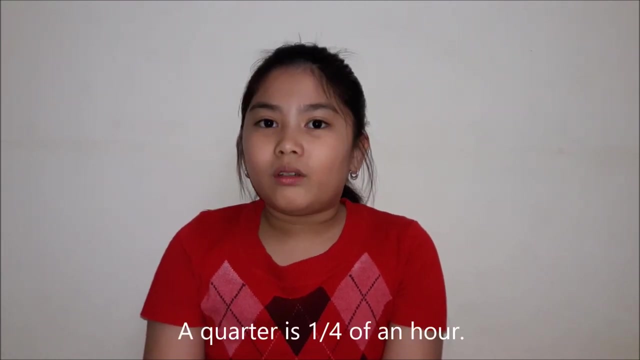 answer as well. what about fractions? we can use fractions in telling the time. each minute is a fraction of the hour, like half past two, which means 2, 30. another example is quarter to five or quarter past four. a quarter is 1, 4th of an hour, so quarter to 5 is 445, which. 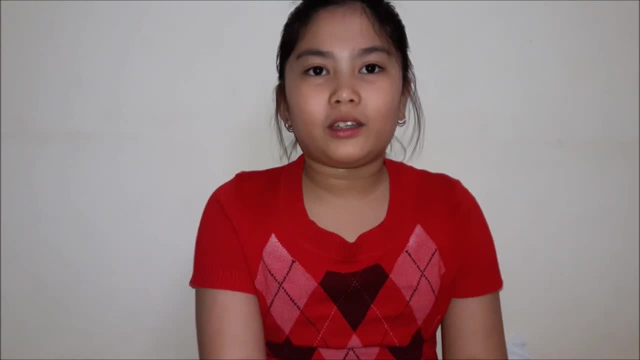 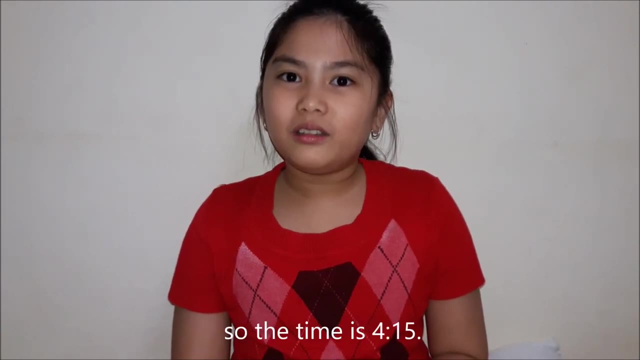 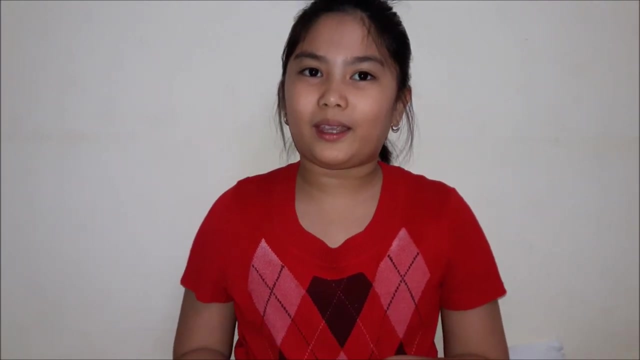 means there's 15 minutes left to 5 o'clock quarter past. 4 means 15 minutes have passed 4, so the time is 4. 15 fractions are also used in cooking, but mostly are used for baking to tell how much of the ingredients we 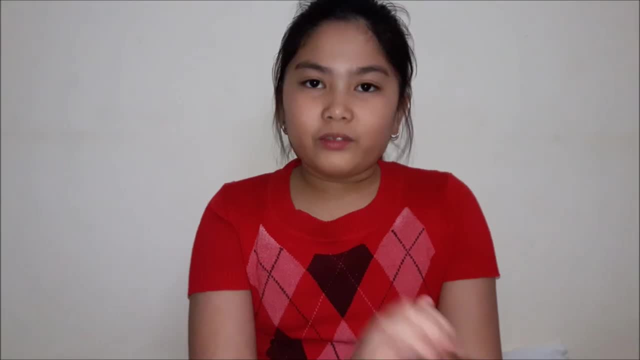 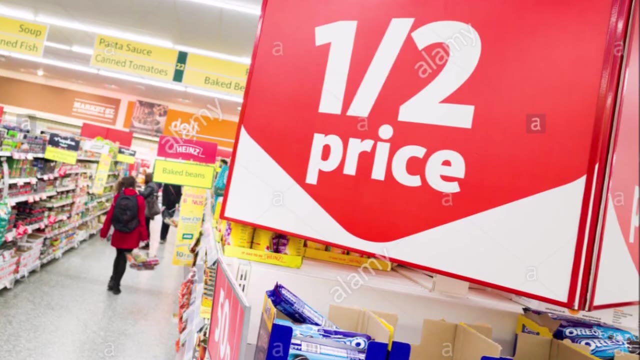 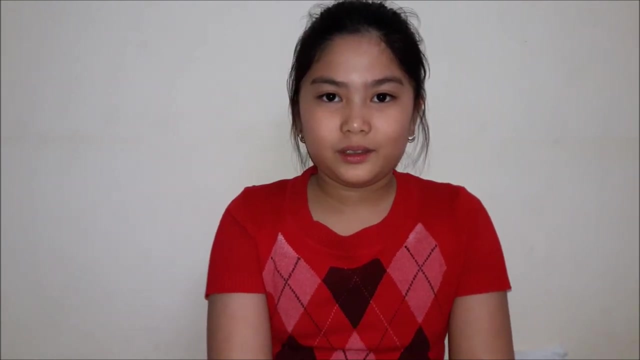 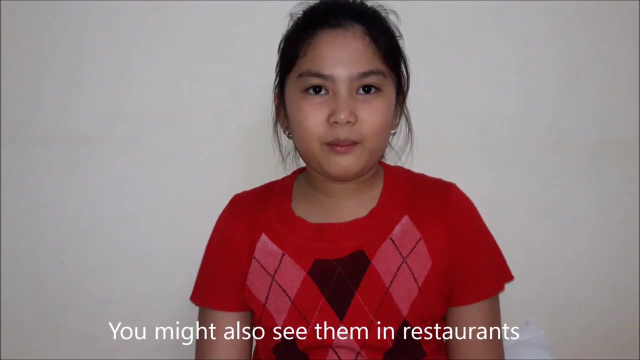 should use. fractions are also seen in grocery or supermarket, such as 1 1⁄2 kilo of fruits, 3⁄4 of meat, 2⁄3 of fish. you might also see them in restaurants, such as when you're eating a slice of. 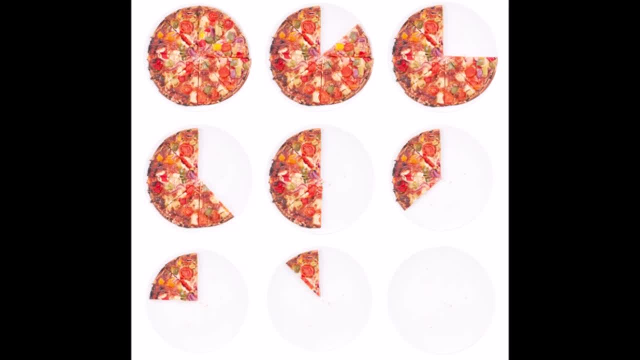 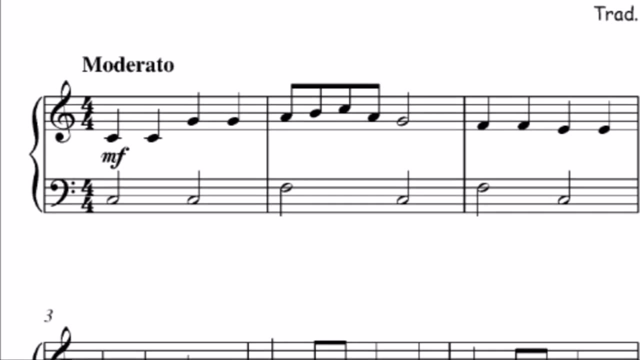 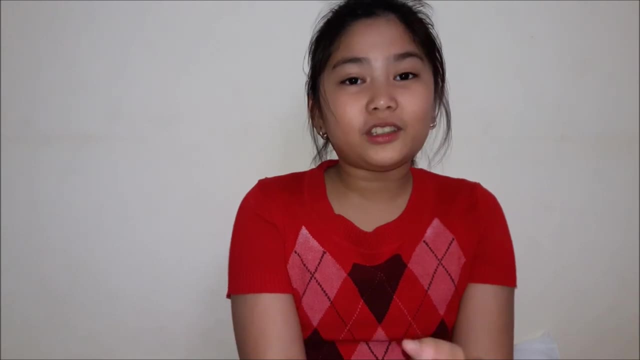 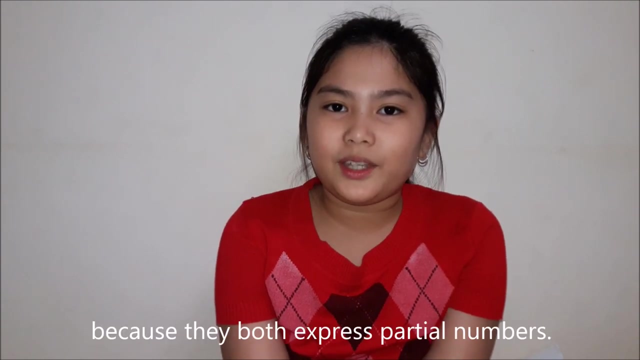 bread or a fraction of a pizza. did you know? music is full of fractions too, it's true. add there a fraction to that too, so this does make sense. There's also a half note, quarter note and a one-eighth note. Fractions and decimals are similar because they both express partial numbers.